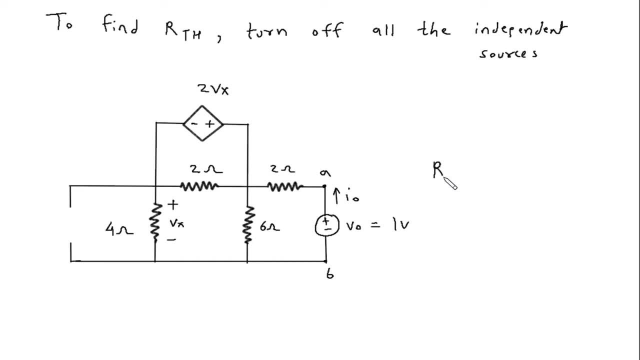 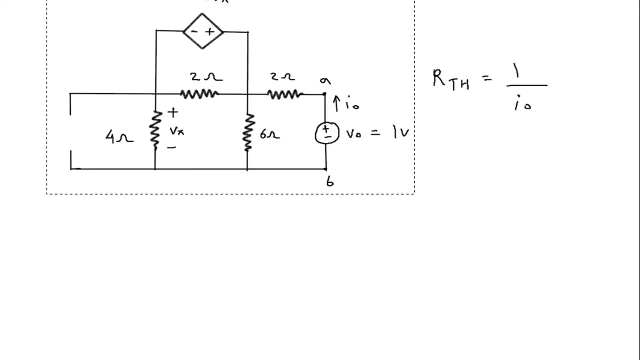 this we can find the value of Rth, like Rth is equal to voltage, which is one by Io. So if we found Io, then from this we can get the value of Rth. So let's find Io, Let's say this is, let's say this is mesh number one with current I1,. 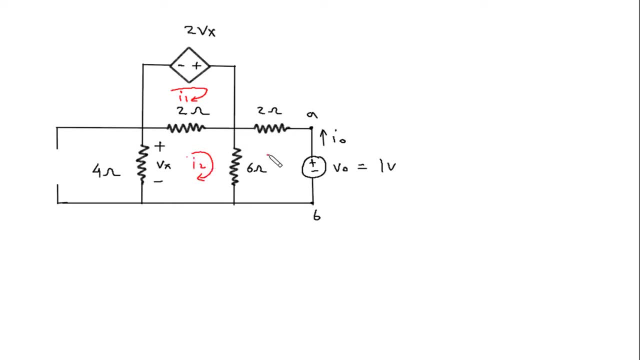 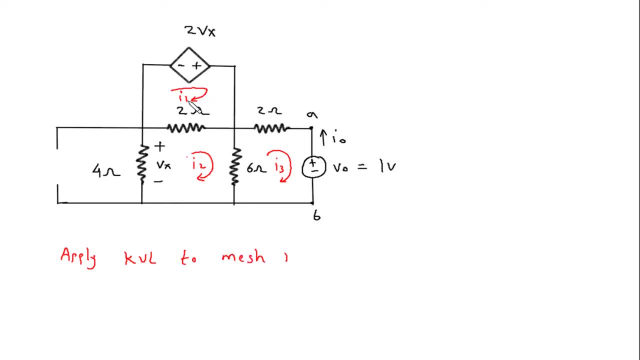 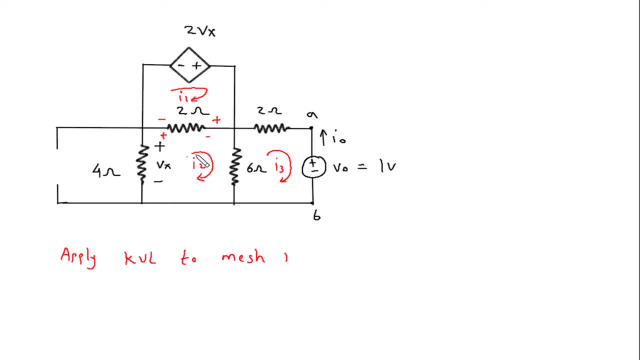 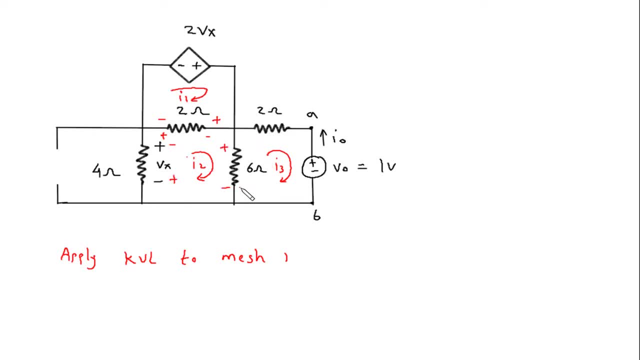 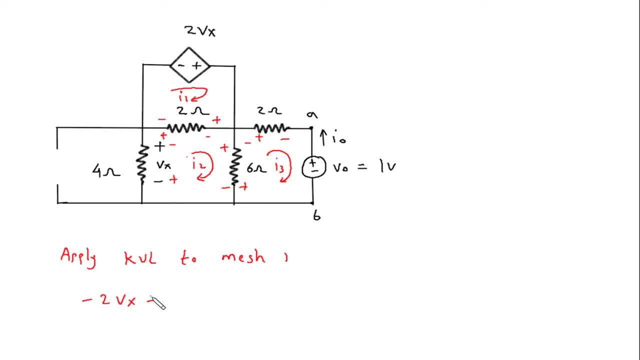 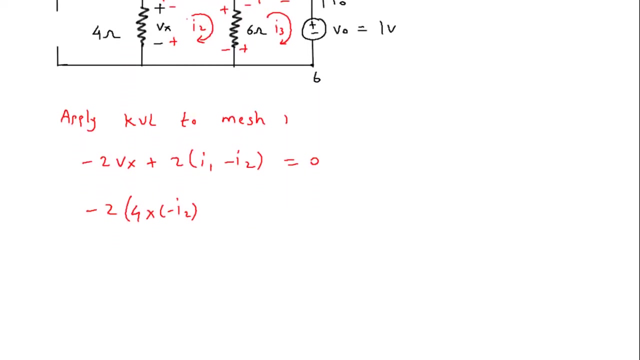 minus 2Vx, then plus 2I1 minus I2, I1 minus I2 is equal to 0, now this will be minus 2Vx is. Vx is 4 into minus 2, because of the polarity, 4 into minus I2, then plus 2I1 minus 2I2 is. 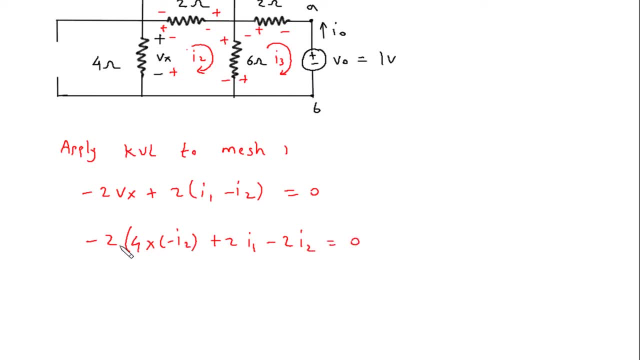 equal to 0, this will be minus, minus plus. this will be 2 into 4, into I1 minus 2I2, this will be 8I2 plus 2I1 minus 2I2 is equal to 0, so this will be 2I1, this will be plus. 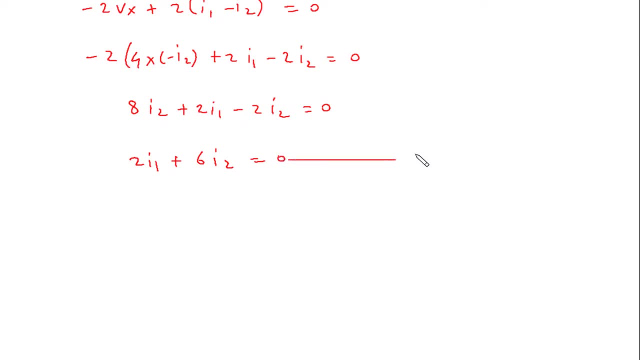 6I2 is equal to 0,. let's say this is equation number 1, now we will apply KVL to mesh number 2, apply KVL to mesh number 2.. So let's say we will start from here. so this will be plus 4I2, then plus 2I2 minus. 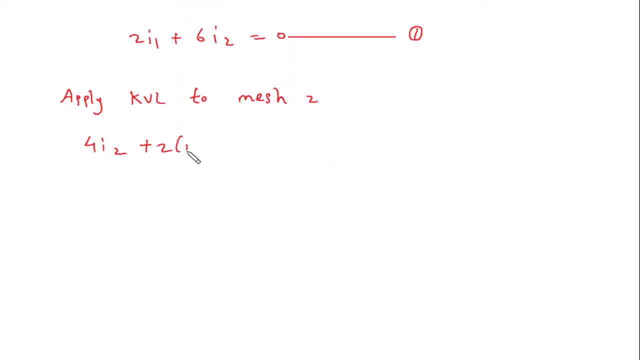 I1, plus 2I2 minus I1, plus 6I2 minus I3.. plus 6 i2 minus i3 is equal to 0.. So this will be 4 i2 plus 2 i2 minus 2 i1. plus 6 i2 minus 6 i3 is equal to 0. 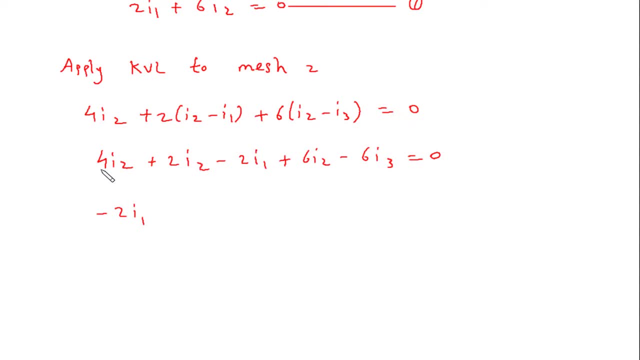 So this will be minus 2 i1.. Then this will be: 4 plus 2 is 6,, 6 plus 6 plus 6 is 12.. So plus 12 i2 minus 6 i3 is equal to 0.. 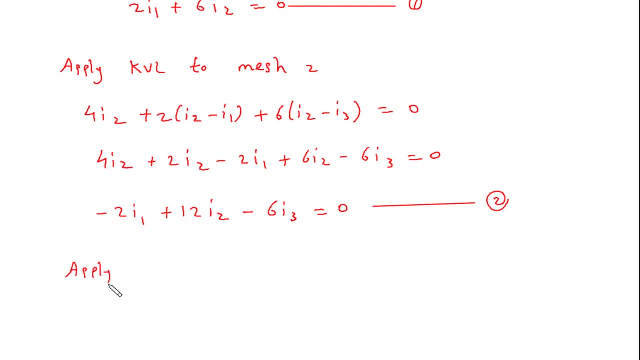 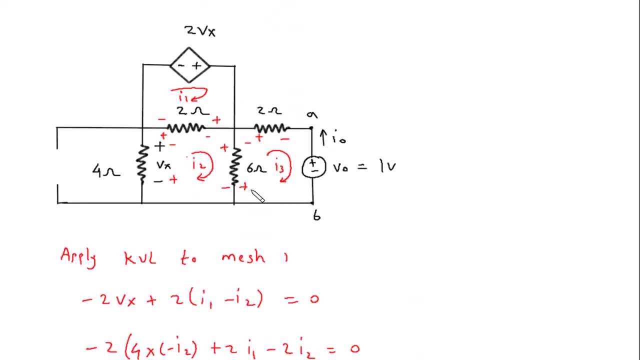 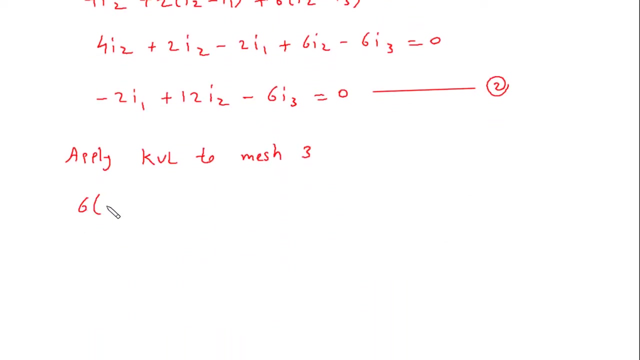 Let's say this is equation number 2.. Now we will apply KVL to mesh number 3.. So let's say we will start from here. So this will be plus 6 i3 minus i2.. Plus 6 i3 minus i2.. 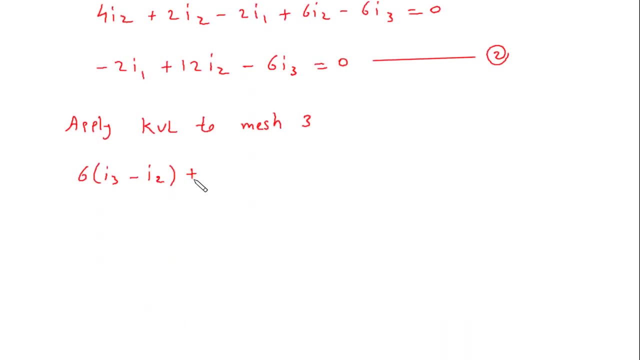 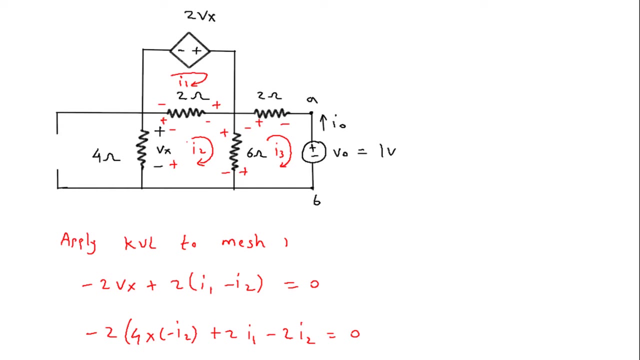 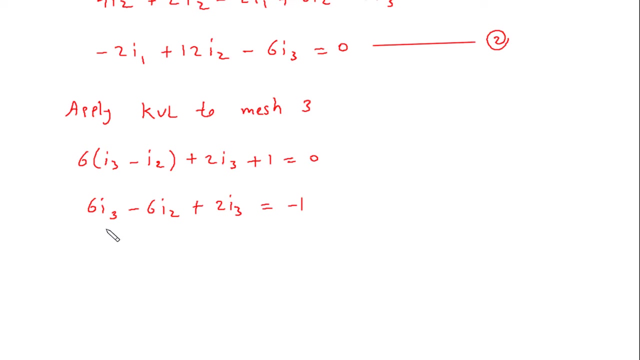 Plus 2 i3.. Plus 2 i3.. Then plus 1 is equal to 0.. Plus 1 is equal to 0. So this will be 6 i3.. minus 6i2 plus 2i3. plus 1 is equal to 0, or directly it is equal to minus 1. so this will. 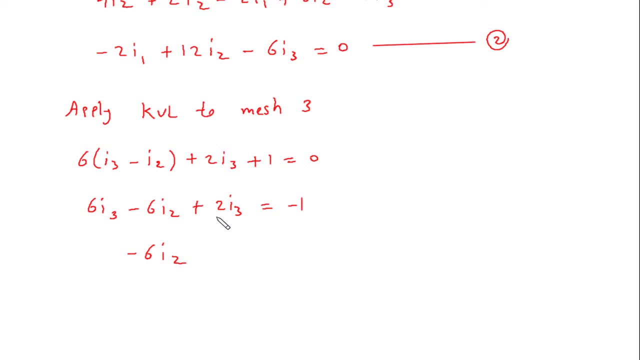 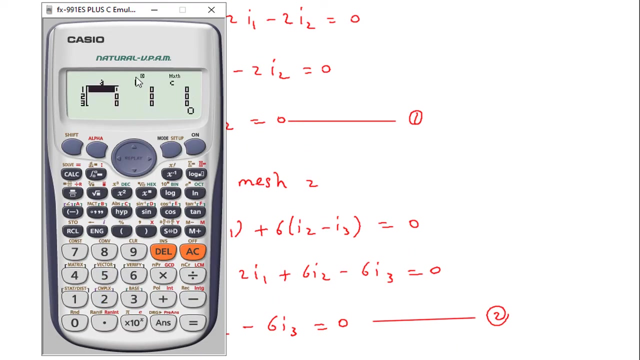 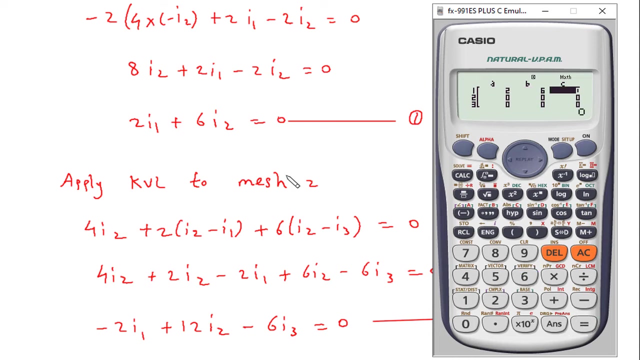 be minus 6i2, then 6 plus 2 plus 8, i3 is equal to minus 1. let's say this is equation number 3. solving equation 1, 2 and 3, we get mod 5, 2, 6, 2, 6, 0, 0. i3 is absent here, so it is 0 then. 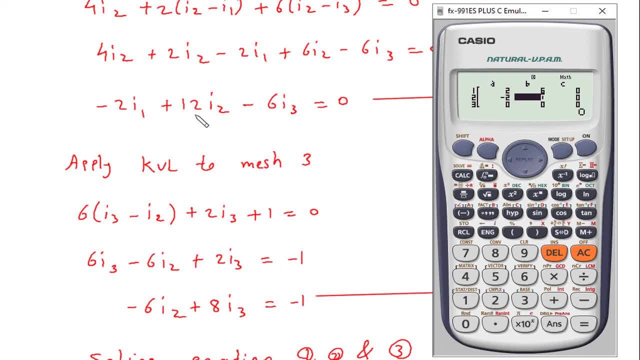 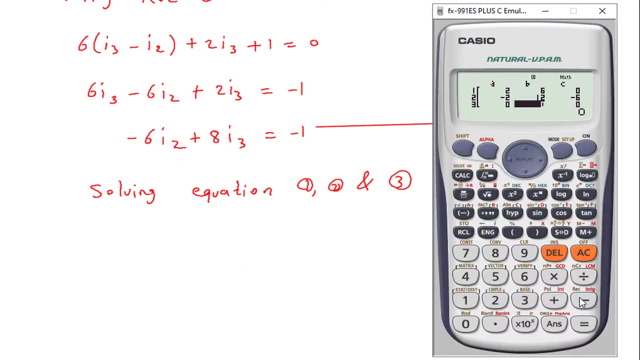 minus 2, 12 minus 6: 0, then from equation 3 i1 is absent. so 0 minus 6, 8 minus 1, i1 is equal to minus 1, 1 by 6. ampere i2 is equal to minus 1 by 18 and i3 is equal to minus 1 by 6. what we have? 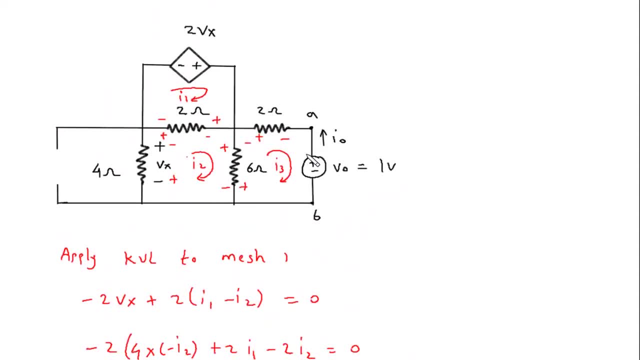 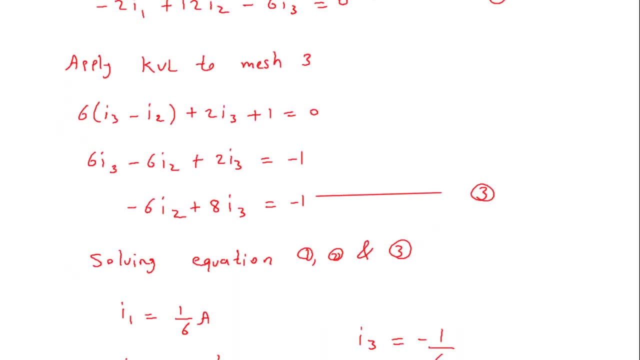 to find. we have to find io. so io is equal to minus io. i3 is equal to minus io. or io is equal to minus i3. io is equal to minus i3, so this is equal to minus minus 1 by 6. so 1 by 6, io is equal to 1 by 6. so we will substitute this value. 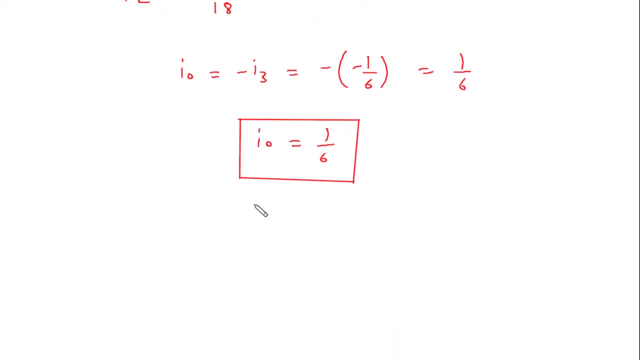 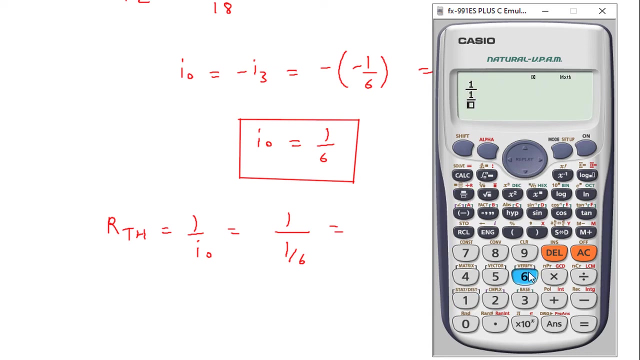 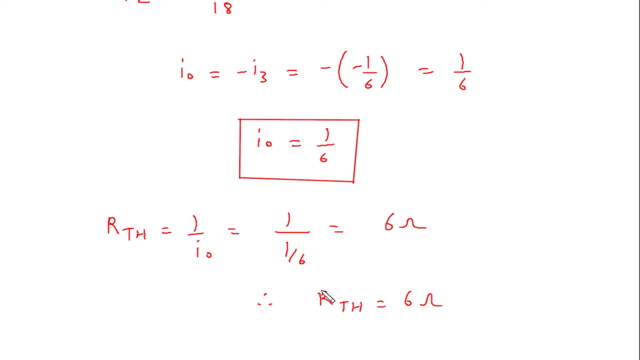 here rth is equal to 1 by io. rth is equal to 1 by io, so 1 by 1 by by 6 is equal to 1 by 1 by 6 is equal to 6 ohm. Therefore Rth is equal to 6 ohm To. 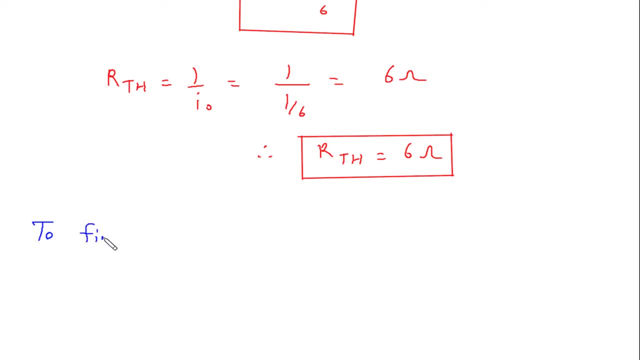 find Vth, to find Vth. so this will be our Vth. This will be positive. this will be negative Here. this will be Vth. Let's assume this is current I1, mesh 1 with current I1. So 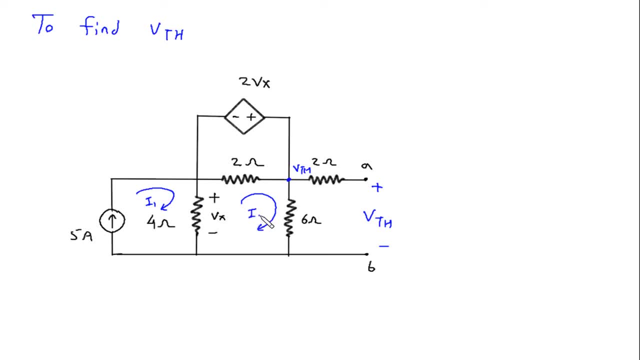 this is mesh 2 with current I2 and this is mesh 3 with current I3.. So, according to the direction of current, this will be positive. this will be negative here. positive, negative here positive, negative, positive, negative here, positive and negative Apply As we can. 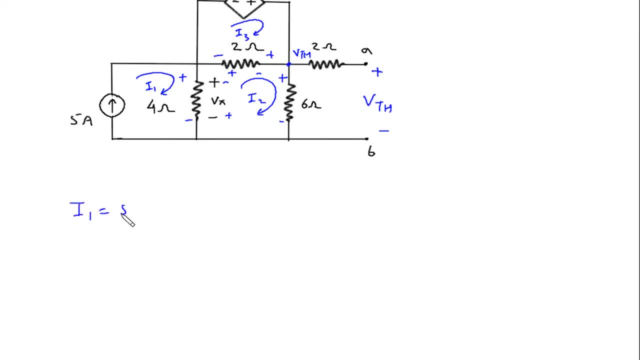 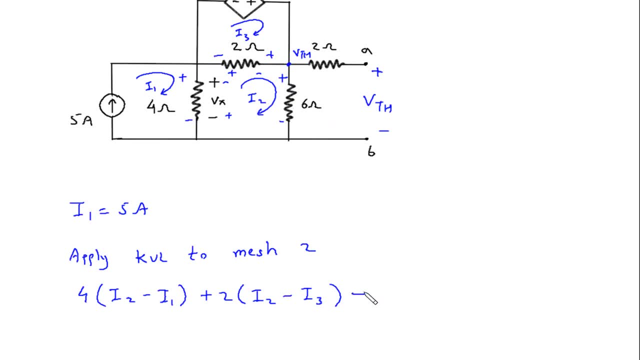 minus I3, then plus 6, plus 6, I2 is equal to 0.. Vth will be equal to this current I2 into 6 ohm, 6 ohm into I2, I2 is equal to Vth. Now we will further simplify this So. 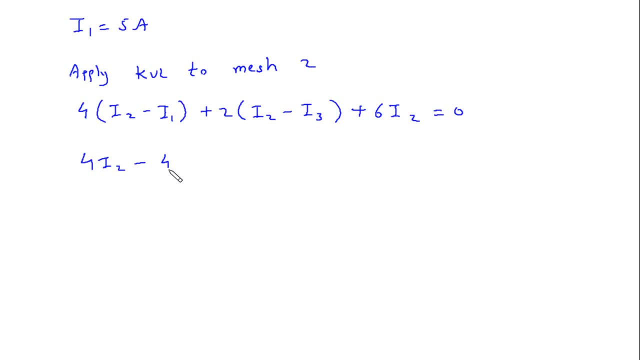 this will be 4, I2 minus 4 into I1.. I1 is 5A, Then plus 2, I2 minus 2, I3 plus 6, I2 is equal to 0. So this will be 4 plus 2,, 4 plus 2, 6.. 6 plus 6, 12.. 12, I2 minus 2,. 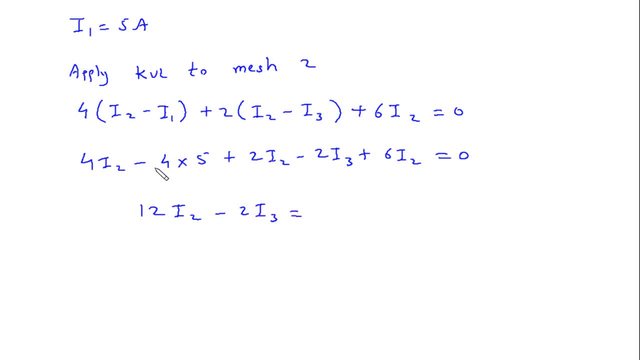 I3 is equal to this will be 5 into 4, 20.. So it's positive plus 4, plus 5 plus 4, I2, minus 4, 6, I1.. This is positive plus 6.. So it will be 5 plus 2, minus 12, 12, plus. 12, I3 minus minus 2, I3. I2 minus second decree equals 10.. personality penalty: equal to 10.. herокlerogen: 0,. so negative: 10, positive: 0, positive, 0, 4 minus 9, factors: 0, positive. 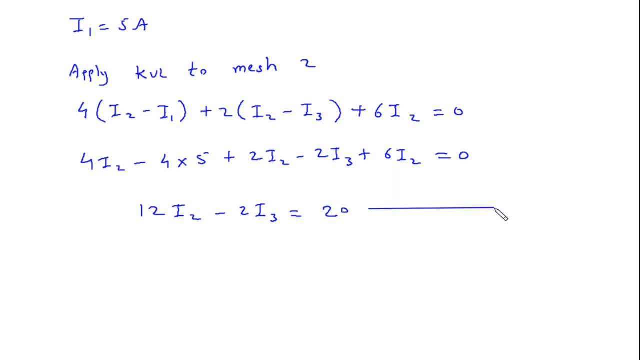 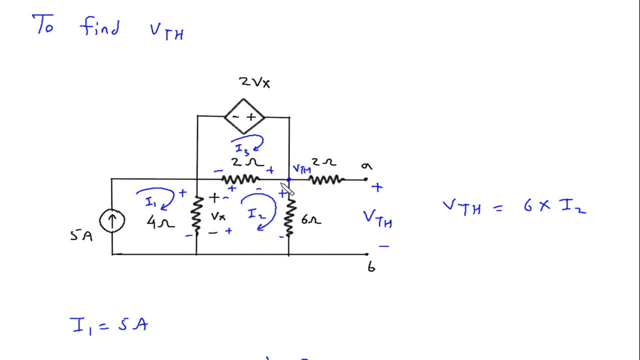 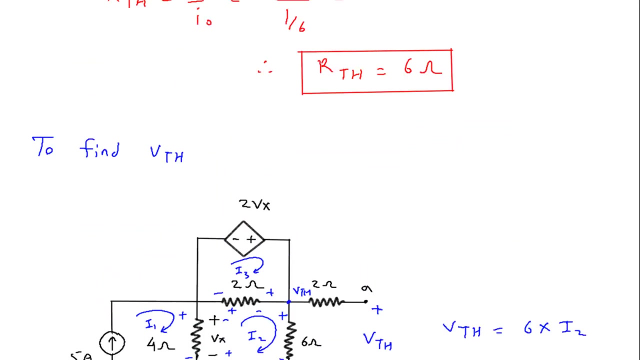 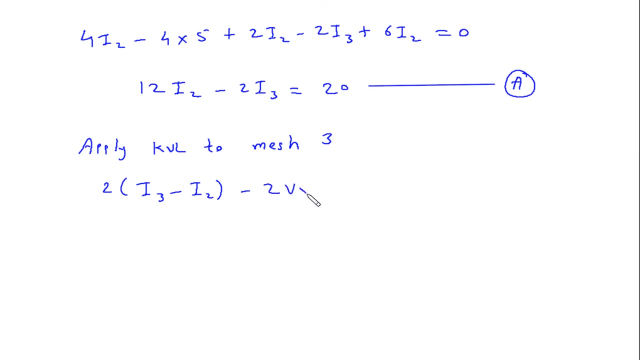 On right side, it will be positive 20.. Let's say this is equation number A. Now we will apply AVL to base number 3.. So let's say we will start from here. So this will be plus 2 I2, I3 minus I2, I3 minus I2 minus 2 Vx minus 2 Vx is equal to 0. 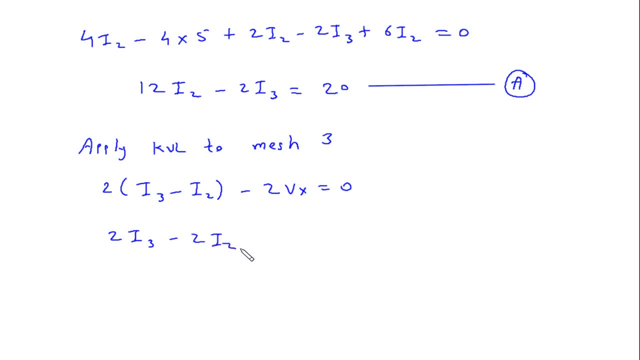 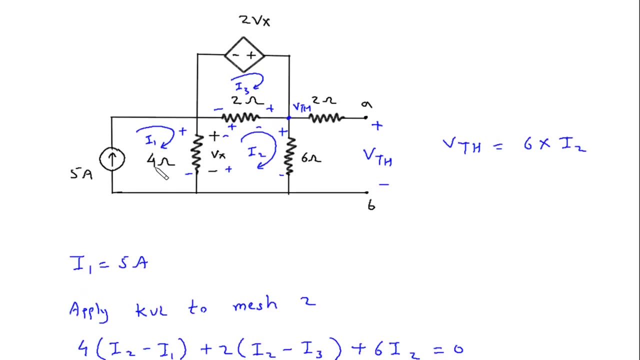 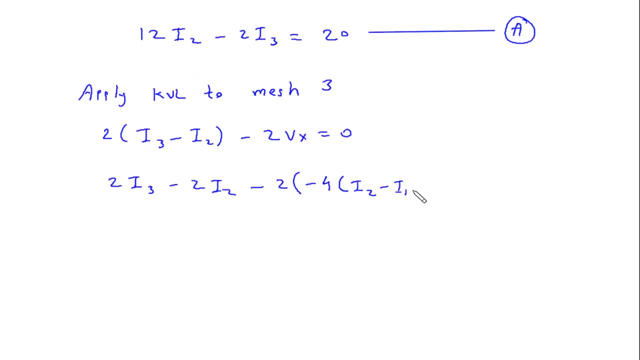 So this will be 2 I3 minus 2, I2 minus 2 into Vx. This polarity is opposite, So this will be minus 4 into I2 minus I1.. Minus 4 into I2 minus I1 is equal to 0. 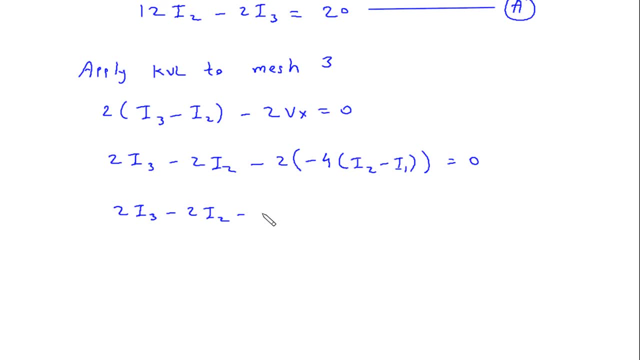 So this will be 2 I3 minus 2 I2, minus minus plus 8 I2 minus 2 Vx minus 2 Vx. This will be minus 8 I1.. Now the value of I1 is given, which is 5, is equal to 0. 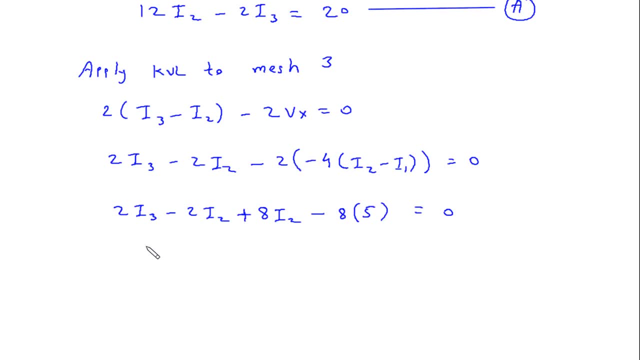 So this will be 6 I2 plus 2 I3 is equal to 40.. Let's say: this is equation number B, Now solving. Let's say: this is equation number B, Now solving. Let's say: this is equation number B, Now solving. 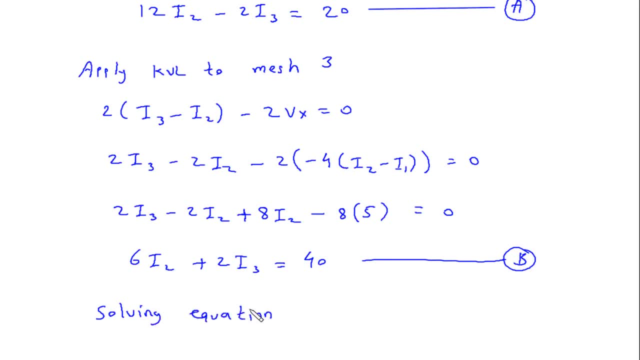 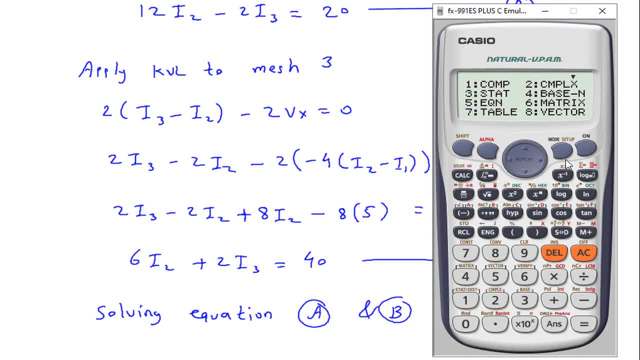 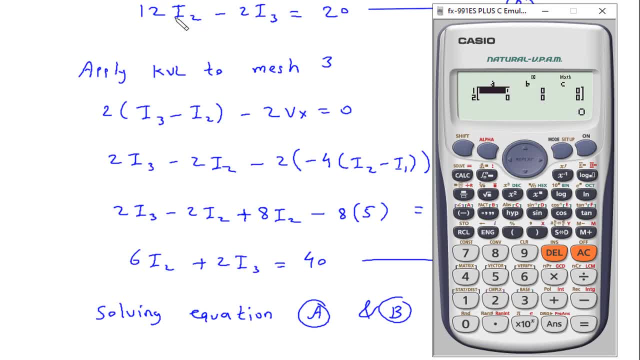